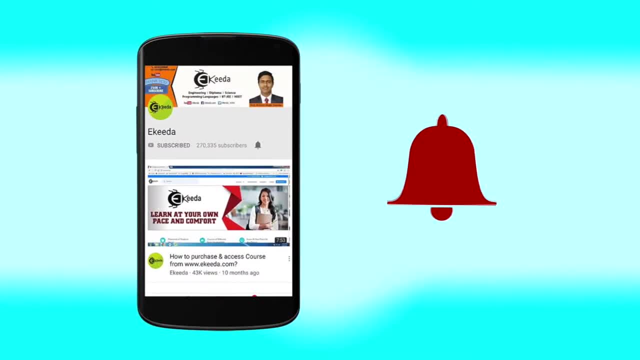 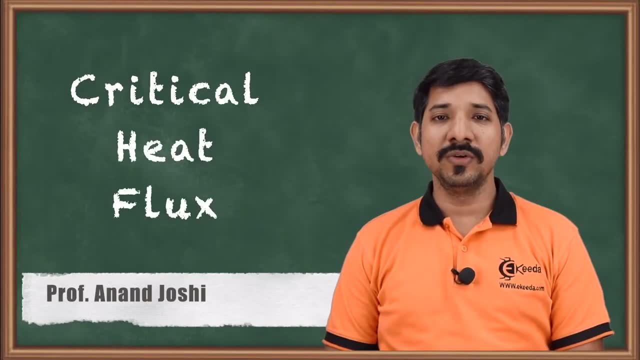 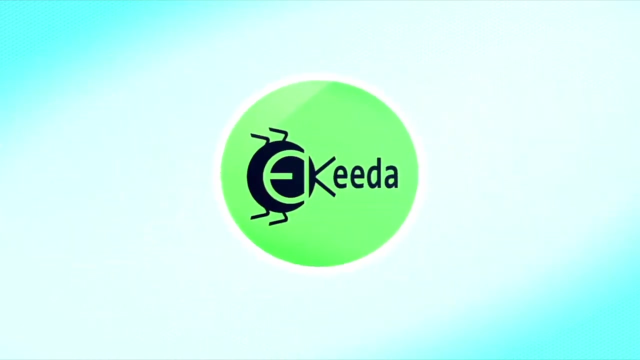 Hello friends, we have talked about boiling and its mechanism. We have also talked about the pool boiling and flow boiling. Now let us talk about a very important phenomena, that is critical heat flux. Now, critical heat flux. So for that we need to first of all understand the Liu-Kiama curve. 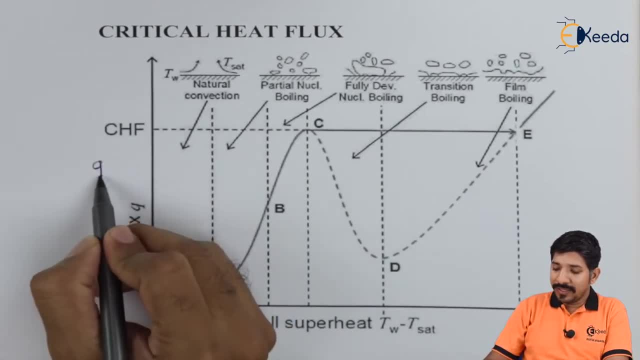 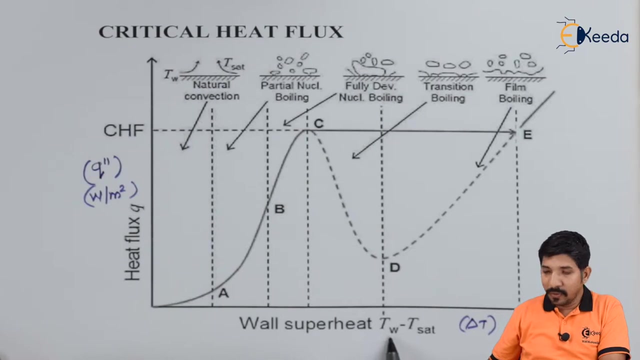 Now the Liu-Kiama curve, basically, is plotted with respect to Q dash. This is nothing but the heat flux which is given in the Watt per meter square to the delta T, Where delta T is nothing but the Tw, Where W stands for wall, So wall temperature minus the saturation temperature, So the difference. 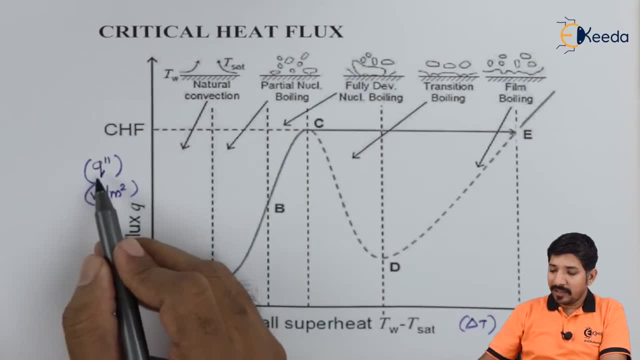 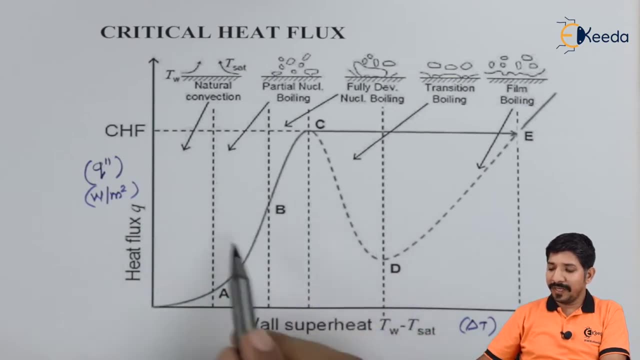 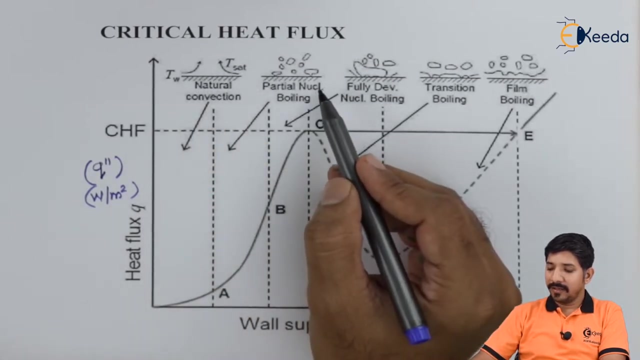 in these two versus the heat transfer flux. If I started plotting the graph, it looks something like this. So we have seen the various regime that is formed in this chapter. The first is natural convection, Then a particular nucleate boiling, Then the fully developed nucleate. 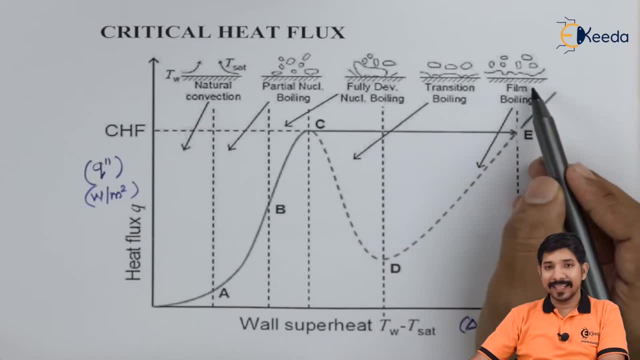 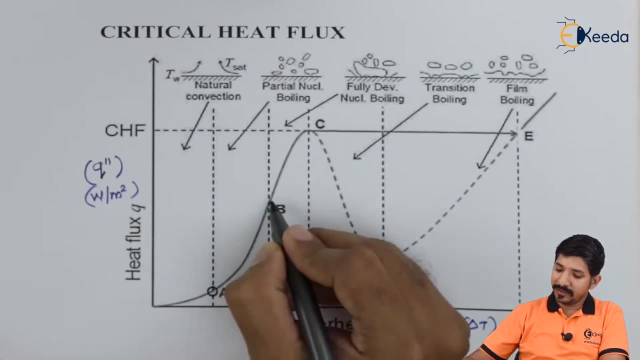 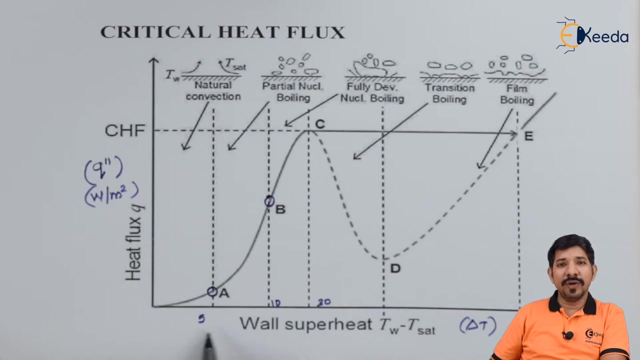 boiling, Then the transition boiling And then the film boiling. Now, in this, if the temperature is between, let us say, 5 to 10 degree Celsius, Then we end up into a partial nucleate boiling Now between 10 to 30. Now this is given when the fluid is water and the wire that we have 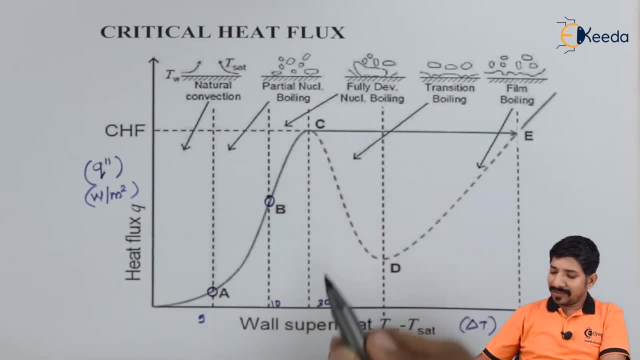 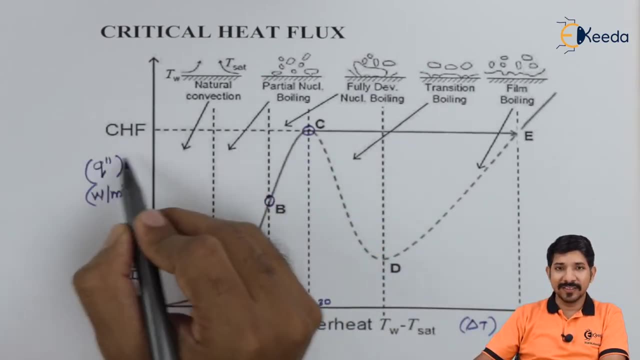 used is the platinum wire. When we have used the platinum wire, When we reach to a 30 degree Celsius delta T, What is happening? We have reached to the maximum heat flux. Now what happens after this? If I, if I may reach to this point, what? 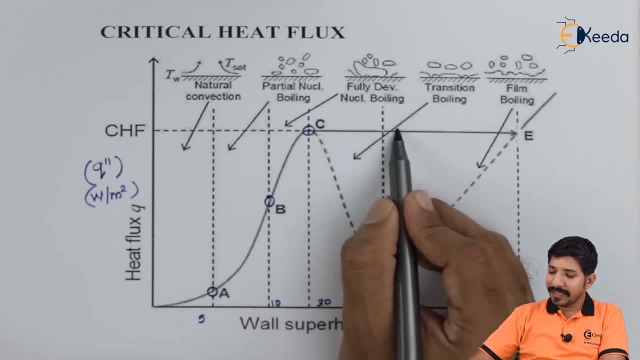 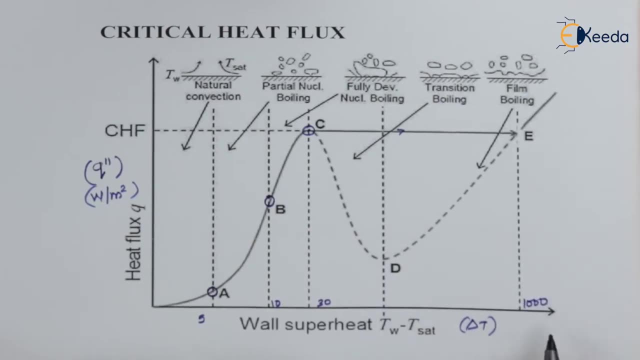 may happen is that the straight away temperature may increase from, let us say, 30 to approximately 1000.. So this, This temperature, This delta T Can be. So let us write down Te. This can be higher than The melting temperature of the wire. 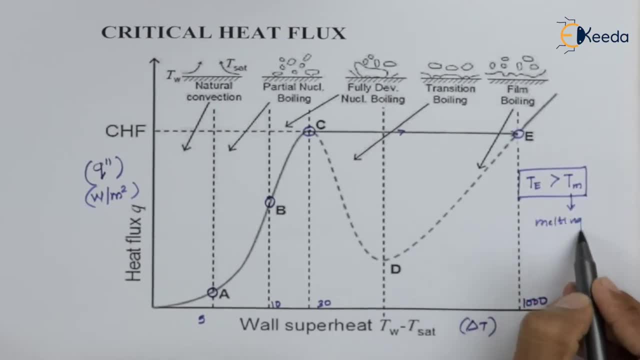 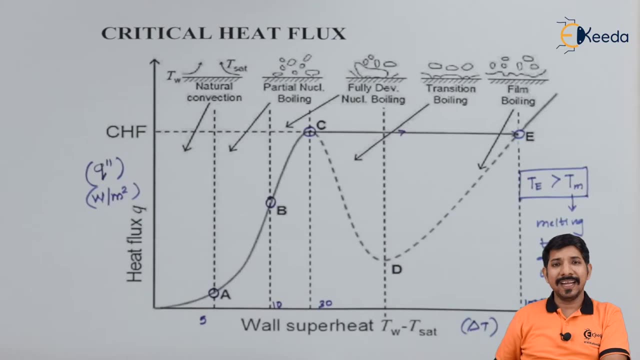 So this is my melting temperature of wire. If we reached this point then there might be a possibility that the melting may have taken Place at a local point. Now, because of this small melting, there might be a possibility thatstaught that change, possibility that this wire itself can be can get broken. so that is why this they 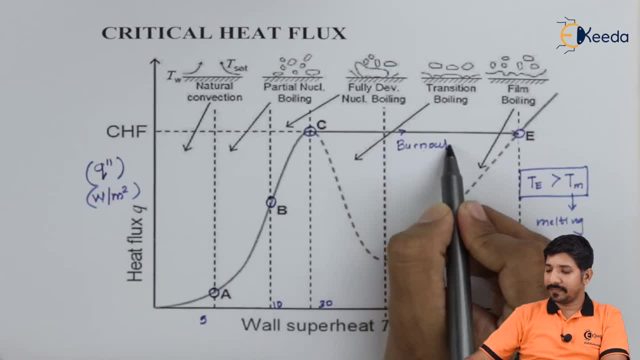 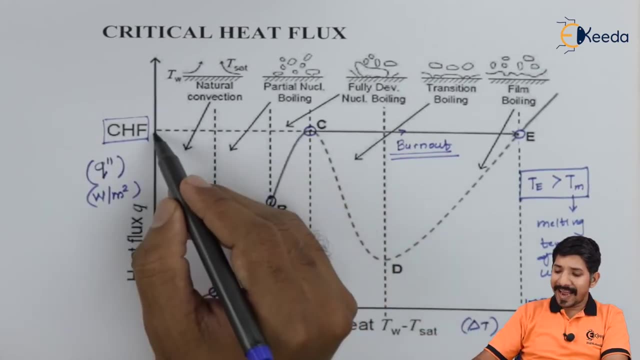 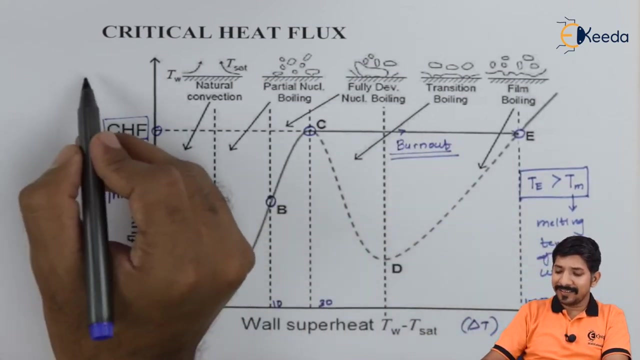 call as a burnout scenario. so the name for the same is critical heat flux, fire. critical because at the this heat flux there is a possibility of burnout of a given wire. so that is why they call this as a critical heat flux. the famous acronym for this is CHF. 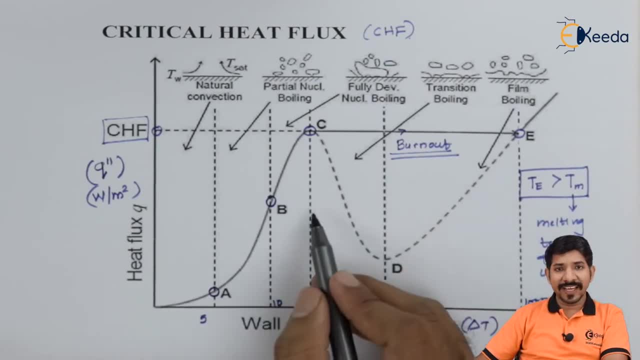 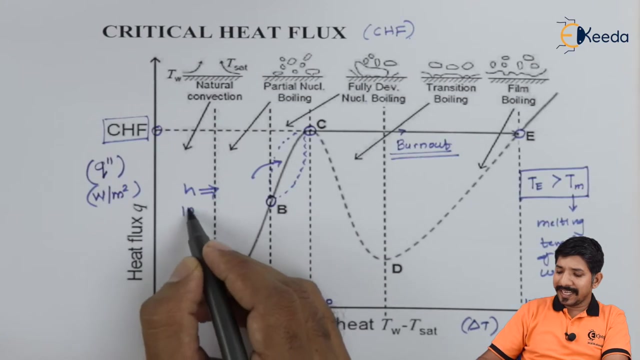 so we really have to emphasize on finding the value of CHF for various scenario. why? because we are always interested in this area. for this area, the value of H is 10 time, 10 time more than any free convection or for convection. so so 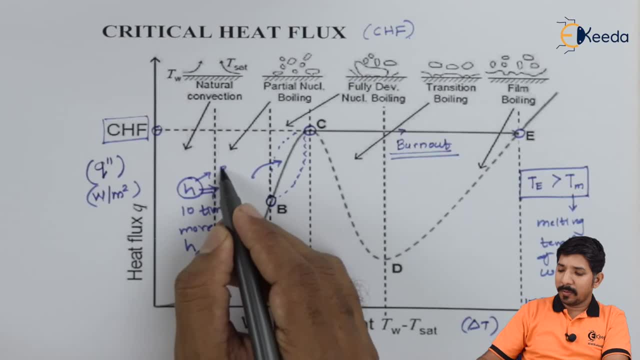 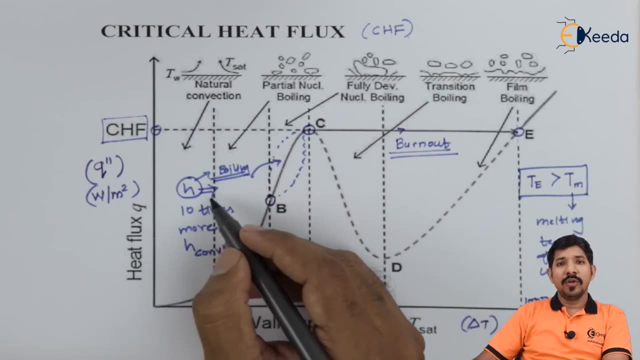 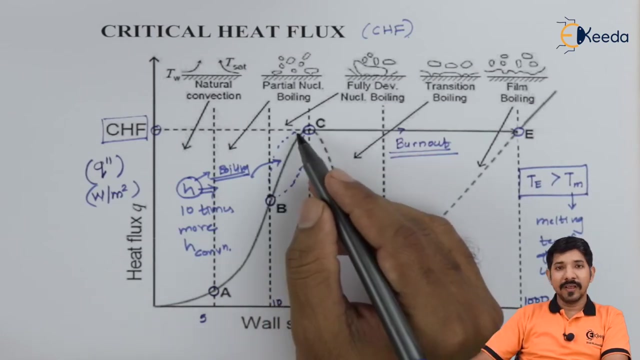 the heat transfer rate by boiling, specifically in case of a nucleate boiling, is quite high. so to have the most efficient heat transfer rate, we try to keep our parameters somewhere in between this. but there might be a scenario that, due to the Delta T, due to slight increase in the Delta T, we may 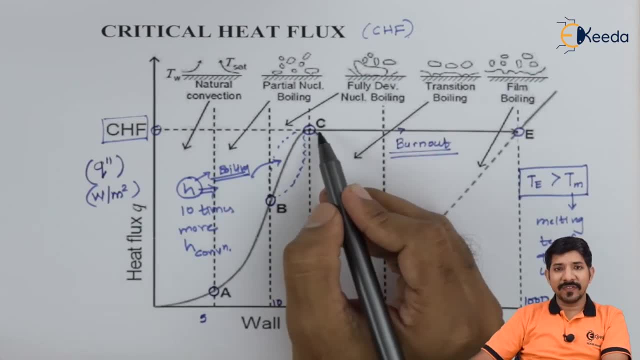 reach to this point. so if we know what is the CHF value for the given fluid combination- fluid and wire combination- then we can make sure that we have not reached to this point. they call this point as a burnout. so basically, there are so many correlations which are available wherein for a given 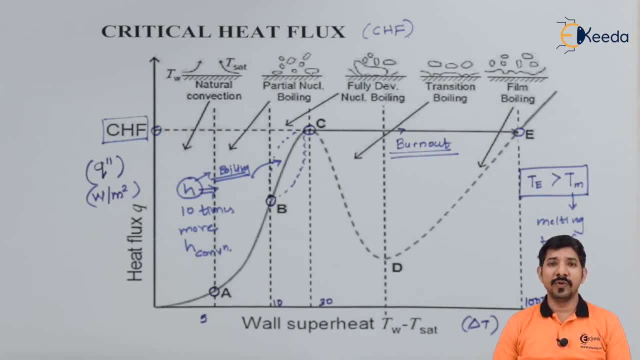 diameter or for a given combination of fluid and surface, the CHF can be calculated. there are so many ways of finding CHF. one is in the empirical correlationship, then second one is by conducting the experiment, then the third one is by various numerical methods, so we can use the CFD equations or basically,